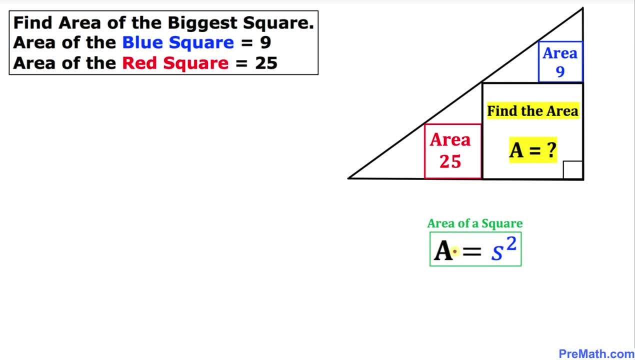 And here is the area of a square, formula A equal to S square, where S is the side of a square, And if we look at this red square, 25 area means that this side is going to be 5, this side is going to be 5 as well, 5 this one and 5 this one, according to this formula. 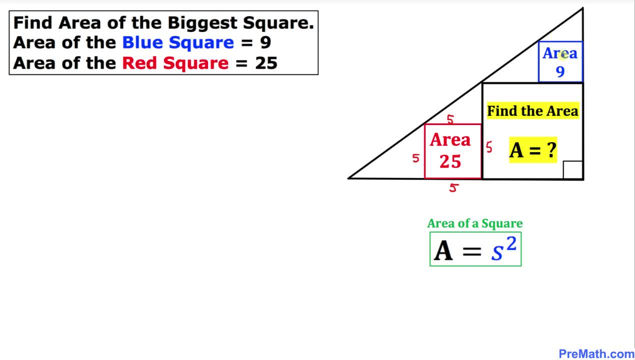 And likewise, the sides of this blue square is going to be 3,, 3,, 3 and 3, isn't it? 3 square is 9 and here, 5 square is 25.. Now, let's focus on this biggest square. We want to find the sides of this big square. 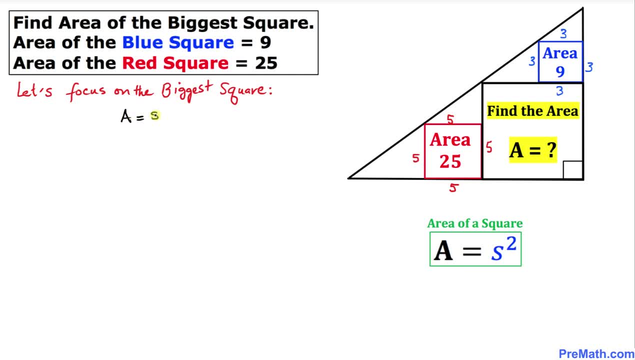 We know that the area is S square. We want to find the value of S. Let's take the square root on both sides. So this square and square root is gone. So that means each side is going to be square root of A. 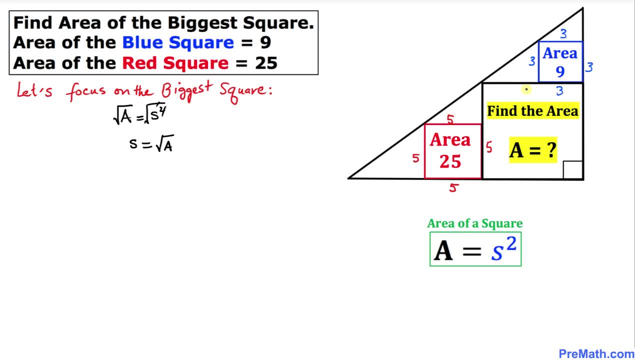 So that means this side is going to be square root of A, this side is going to be square root of A, this side is going to be square root of A and this side is going to be square root of a as well. and in this next step, let's focus on this. 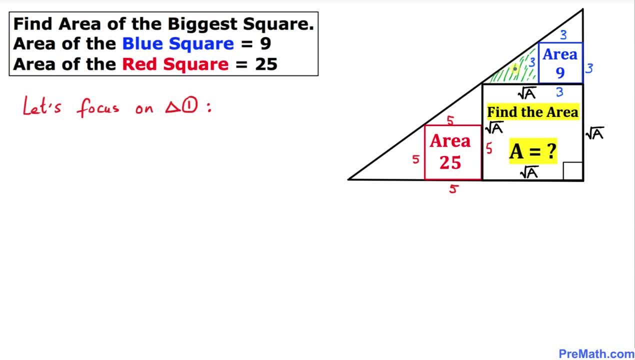 shaded triangle. i am going to call this triangle number one, as we can see that this is a right triangle and, moreover, this side of this triangle number one is three units, and this one over here, the horizontal part that's going to be like this one is going to be, the whole length, is square root. 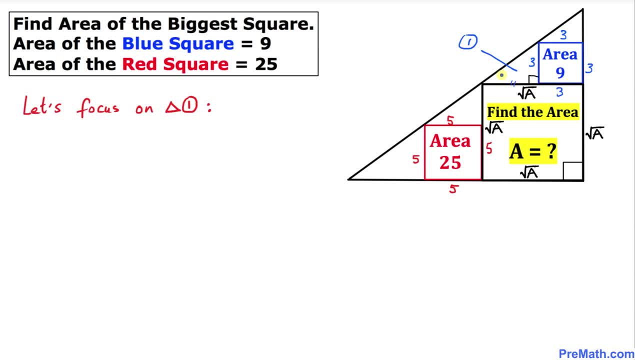 of a and we take away this three, so that is going to become square root of a minus three. now let's focus on this shaded triangle, and i am going to call this triangle number two, and, as we can see, that this triangle is also a right triangle and, moreover, in this triangle number two, the horizontal, 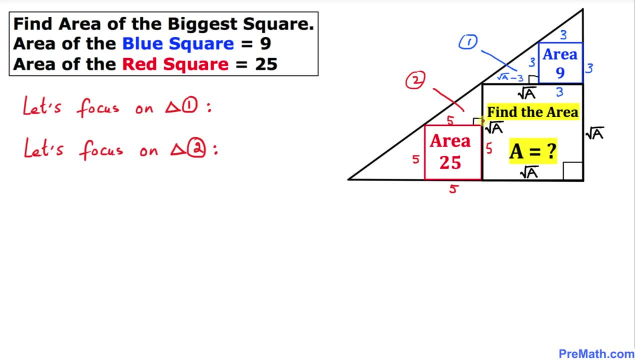 side is five units. and now we want to figure out the vertical side and we are going to call this triangle number two and as we can see that this triangle is also a, that is going to be we know the whole. this length is square root of a take away five. so that is going. 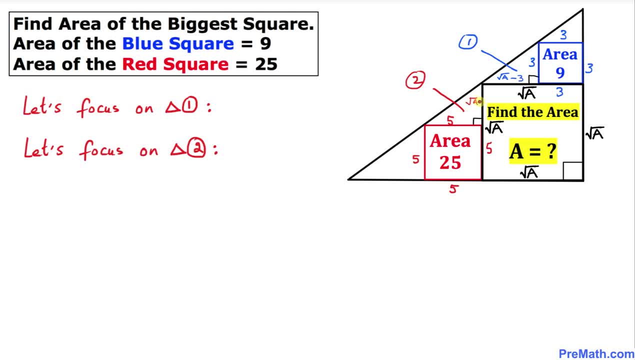 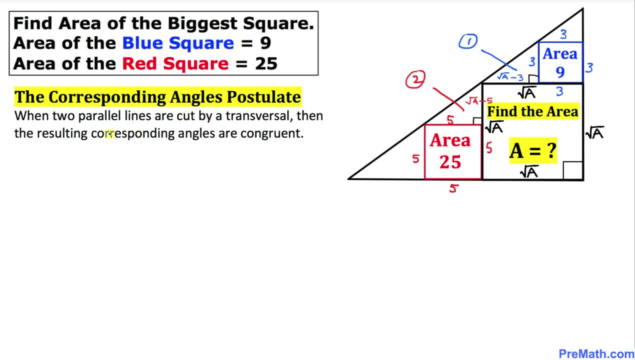 to become square root of a minus five. and here is our corresponding angles postulate. and also look at these angle: this angle in this triangle and this angle in this triangle, and they are corresponding angles and, according to this postulate, they are congruent. likewise, this corresponding angle: 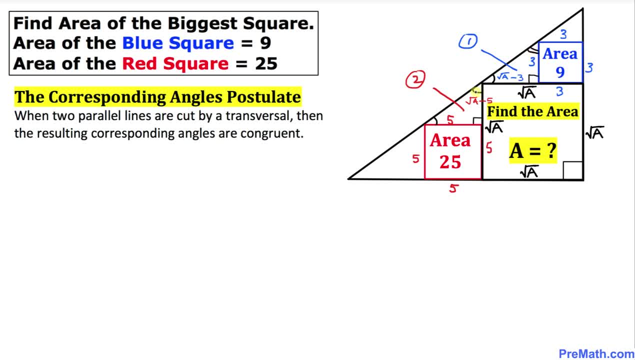 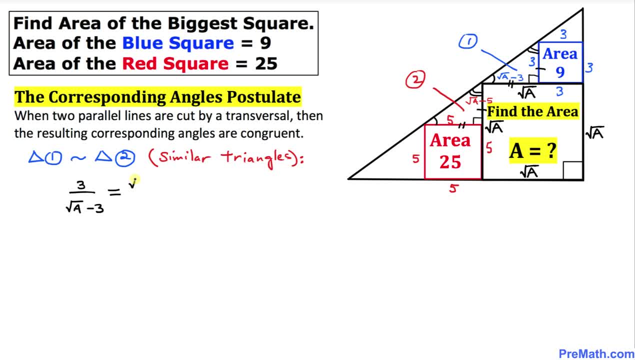 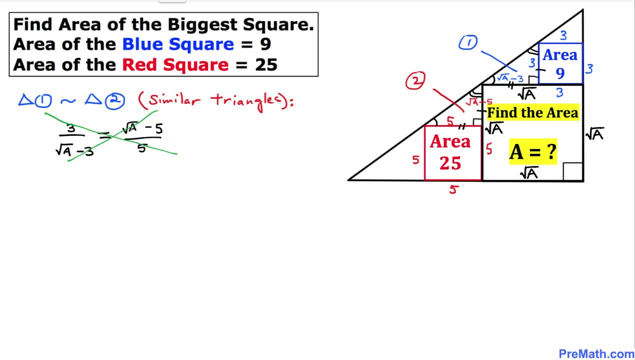 this side, which is square root of a minus 5 divided by 5. now let's go ahead and solve for a. let's crisscross first. we're going to cross, multiply, and let's go ahead and do this one that is going to give us: 3 times 5 is 15, equal to when we multiply the other way around, we have a. 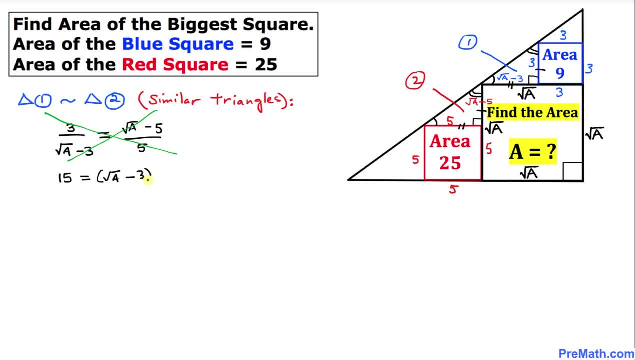 square root of a minus 3 times square root of a minus 5.. and let's go ahead. and now, on the right hand side, let's use a foil method. we're going to twice, so this time this, and then this time this, and then, finally, this time this. let's go ahead. 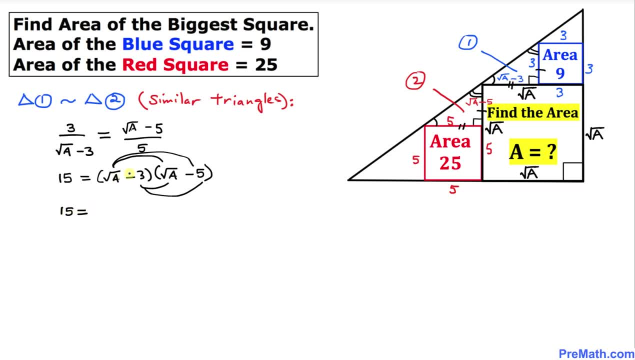 15 is on the left hand side and the right hand side. when we multiply this thing, this is going to be square root of a times square root of a, minus 5 times square root of a, then minus 3 times square root of a and then finally negative 3 times negative. 5 is going to give us positive. 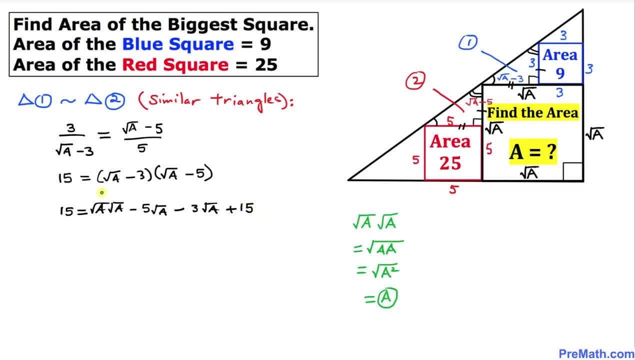 15 and over here. as you can see, square root of a times square root of a is equal to a, according to this explanation. so I can write this one: 15 equal to a, and then we let's combine these like terms. that's going to give us negative 8 times square root of a plus negative. 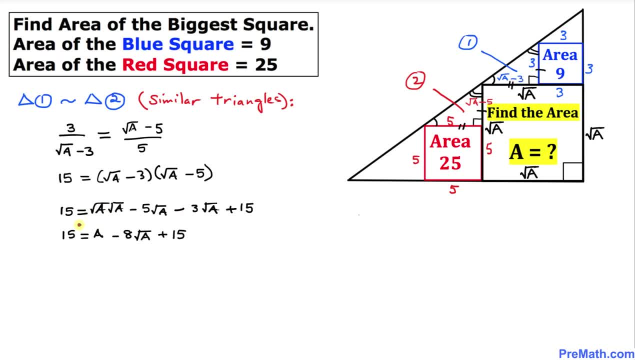 15 and now, as we can see, we have a 15 on this side- left side- and positive 15 on this side. they cancel each other out, so we ended up with zero equal to a minus a times square root of a, which could be written as a equal to a times square root of a.